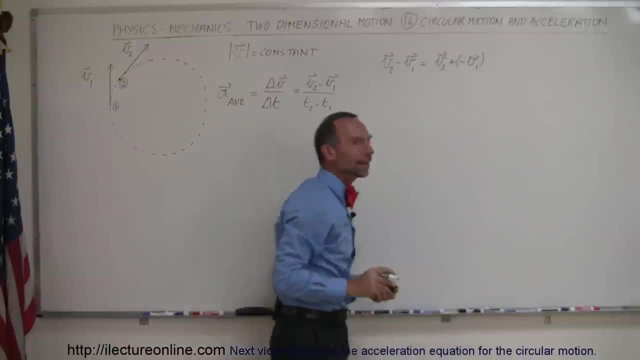 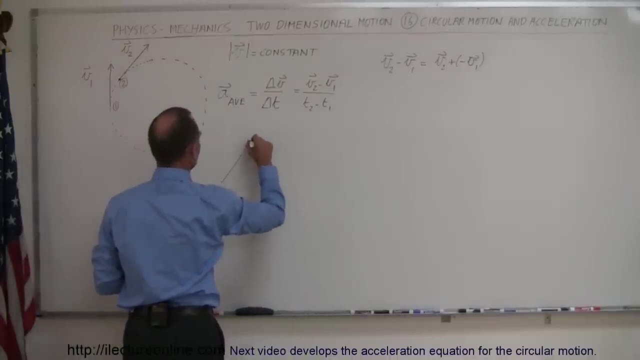 plus the negative of v1. so let's go ahead and do that. let's add v2 and the negative of v1. so here we have v2, and v2 looks like this: this is our v2 vector. now we're going to add to that the. 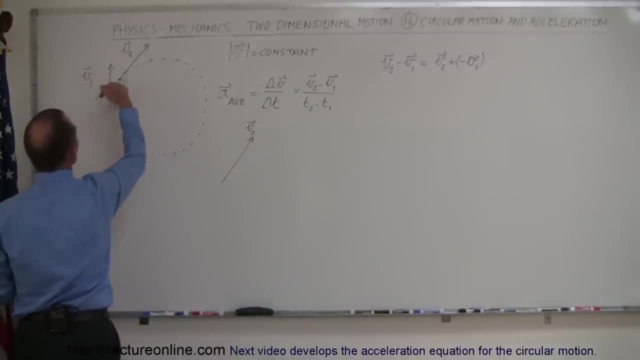 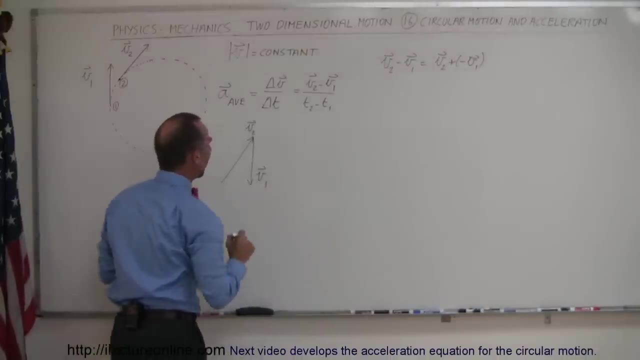 negative of v1. since v1 points directly upward, we're going to turn that around and have a point directly downward. so there is v1 and i'm assuming very small angles. of course i made the angles here bigger so it's easier to see, but i'm assuming very, very small angles. so you can see that if i add. 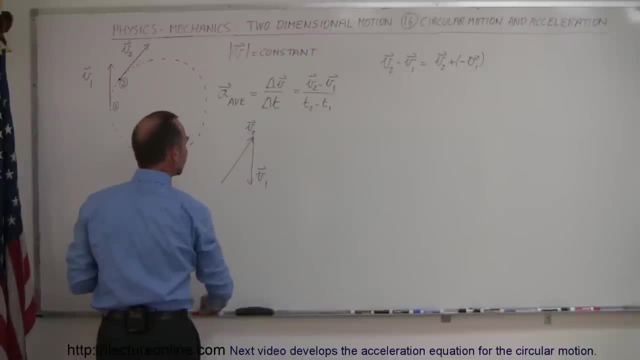 these two together, the side and the lift will be very, very small. so if i add these two together, the sum of V2 and the negative of V1, so this is actually the negative of V1, so that becomes this vector, right there, So this vector can be represented by V2 minus V1.. Notice that. 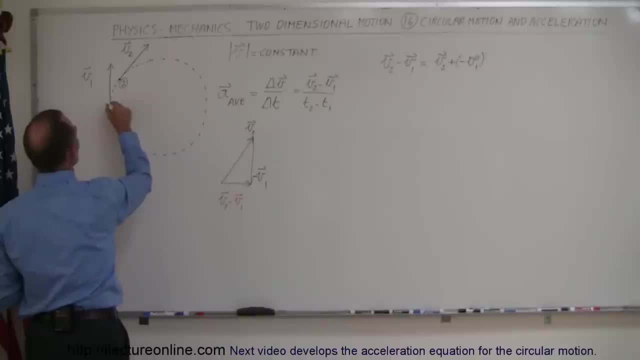 vector points directly to the right from this location right here. so actually it points perpendicular from the path or the circular path right there. so this is here V2 minus V1.. And then if we divide that by the time, now the time is simply a scalar quantity. 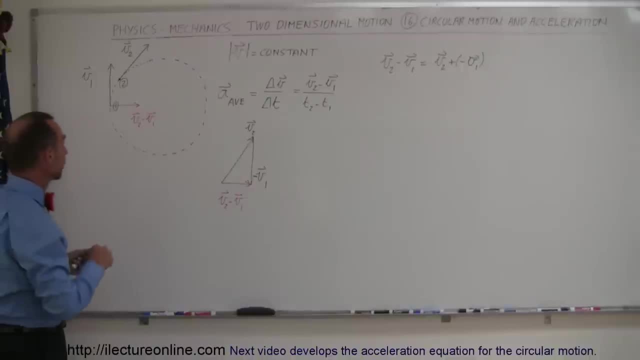 so that can be large, that can be small. If it's small, of course it goes rather fast. If it's large, it goes rather slow. but it doesn't matter. If the object goes really fast, then delta T will be very small. If I divide this by a very small number, I will get a very small number. So if I divide this by a very small number, I will get a very small number. So if I divide this by a very small number, I will get a very small number. So if I divide this by a very small number, I will get a very large vector, meaning I. 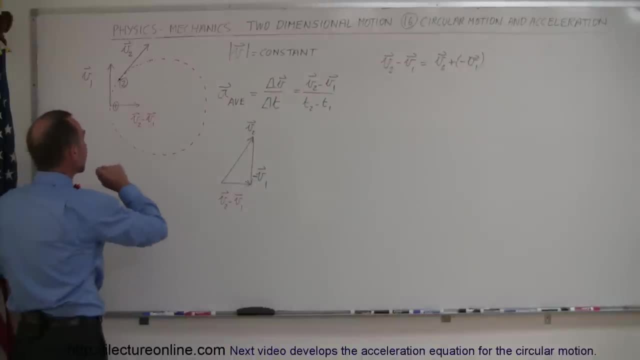 have a large acceleration. But if the object is moved very slow and the delta T will be very large, then of course I divide by a large number and then this vector will become very small. So this is the acceleration vector. It's not equal to this, The acceleration. 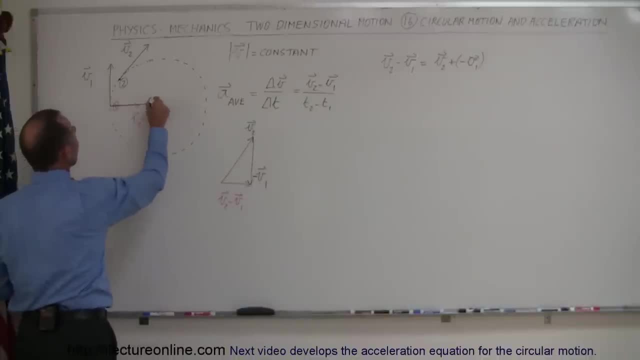 vector would be, let's say, equal to this, That would be the acceleration vector, because the acceleration vector is pointing in the same direction as this V2 minus V1, but it's also divided by the difference in the time between those two points. So, again, if this,